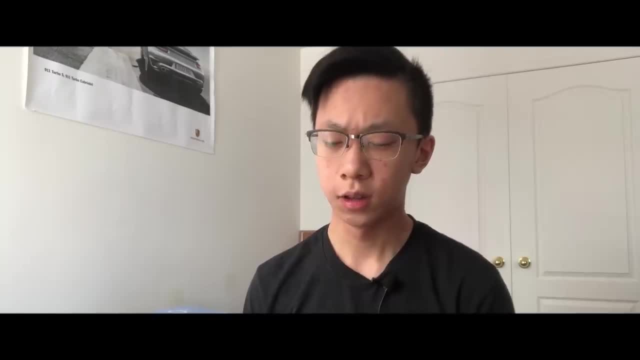 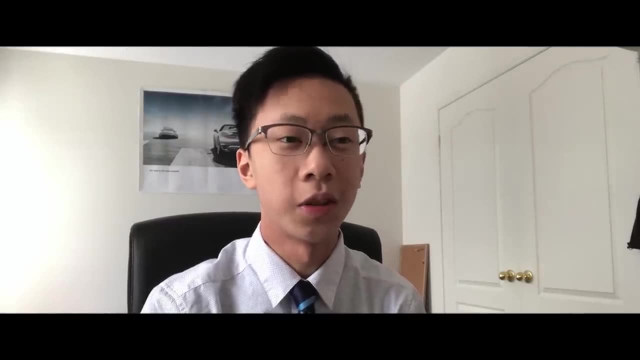 but it's a bit slow. As you mentioned, it's quadratic in time. Do you think you could make it even faster? Of course I knew this was coming. Yeah, so we can just sort the array first and then use a left and a right pointer and move those towards the middle of the array. 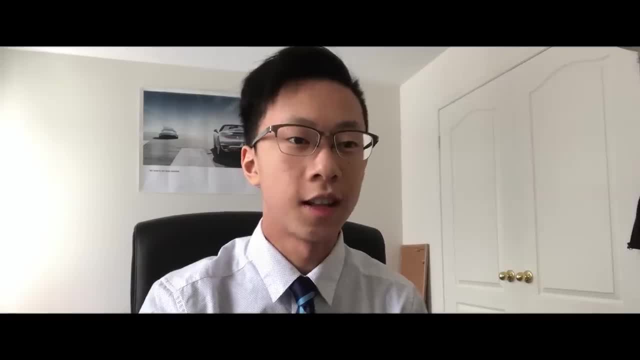 accordingly, based on whether the sum is less than or greater than our target, And so the time complexity of this solution would be O of n log n, because we need to sort the array and then we also have just one pass through the array, which is O of n. 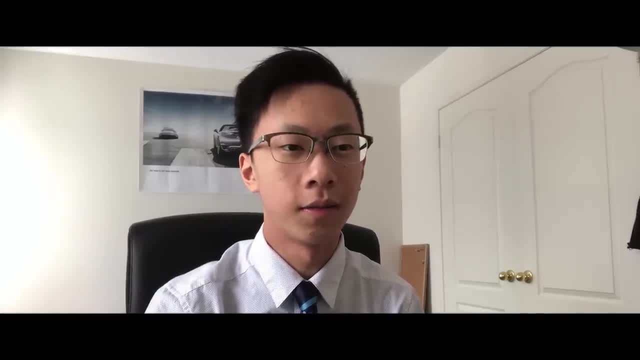 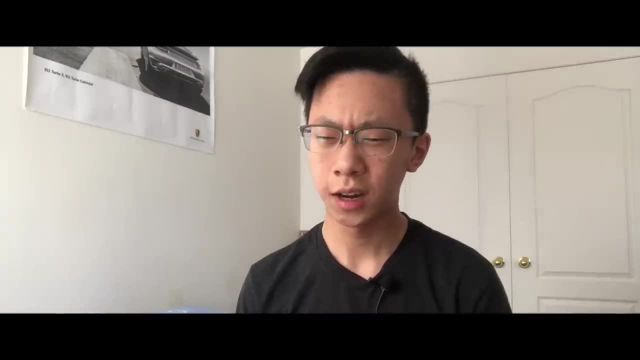 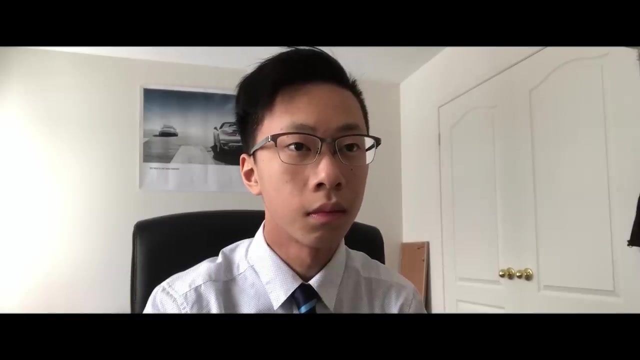 and also our space. complexity will be O of 1.. Yes, I did it. I definitely passed the interview. Well, yes, this is a bit better, but it's still kind of slow. I want you to think of a solution in linear time. What Linear time? I thought I already got the optimal solution. 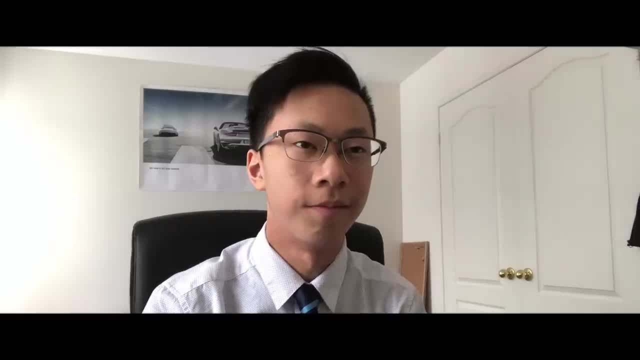 There's no way you can make it even faster. Hmm, Uh, well, I uh, I guess we, we could uh. maybe uh instead of doing, uh what we had before. we could uh instead, uh, do. 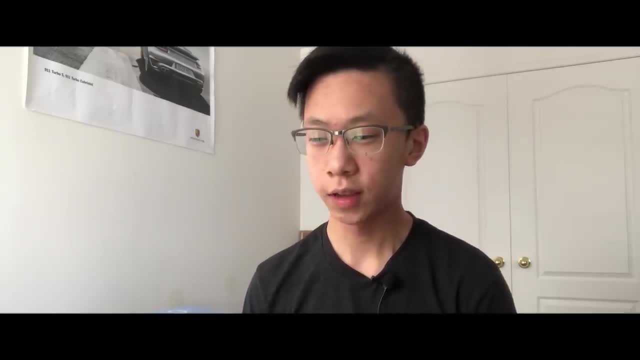 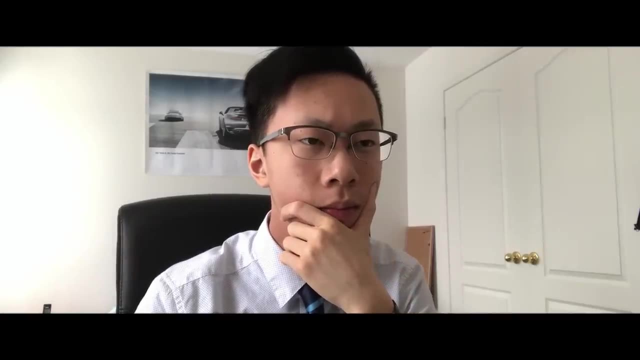 uh, uh, Nick, we only have about five minutes left, so if you can't think of a better solution, don't worry about it. Come on, Nick, Think, Think. What could we do? Man, I'm so stuck. 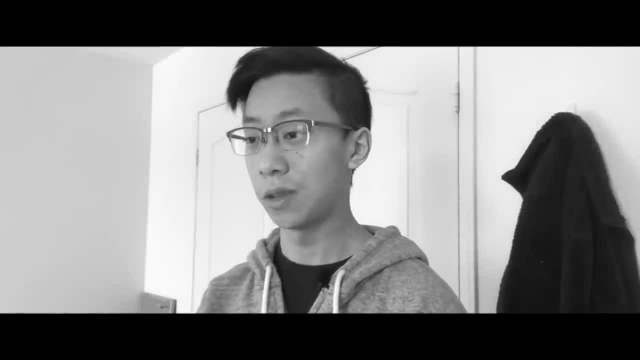 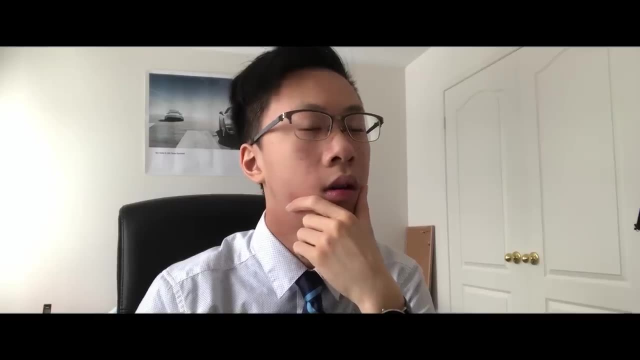 Wait, Stuck, If you ever get stuck, just throw a hash map at the problem. Throw a hash map at the problem. Hash map, hash map, hash map. That's it. I'll use a hash map. Yeah, so we can use a hash map. 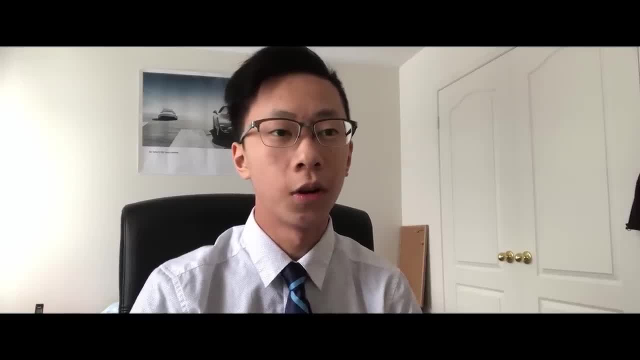 We can just iterate through the array and find the complement of each number, And if the complement already exists as a key in the hash map, we can just return the corresponding, which is going to be an index along with our current index, And the sum of the two numbers at those indices will add up to our target. 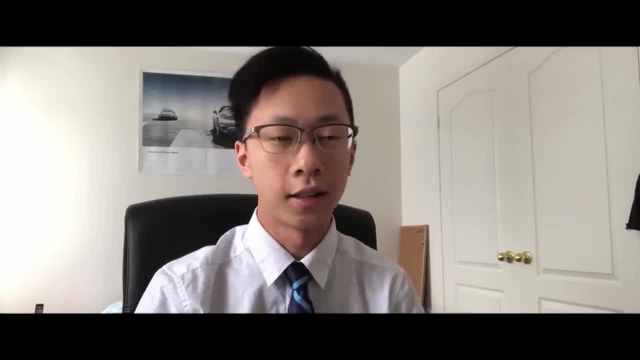 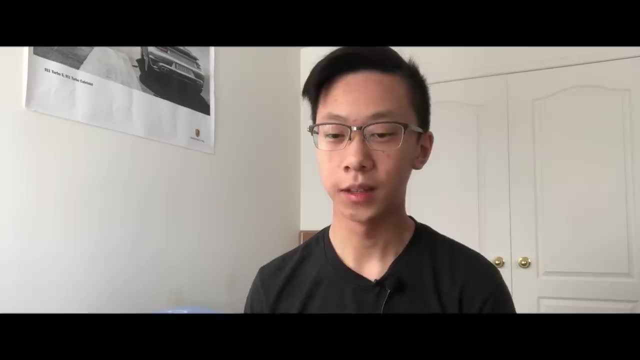 And if the complement does not already exist as a key in the hash map, then we're just going to store our current number along with our current index in our hash map. Yup, That sounds like a pretty good plan. Um, we only have a few more minutes, though.